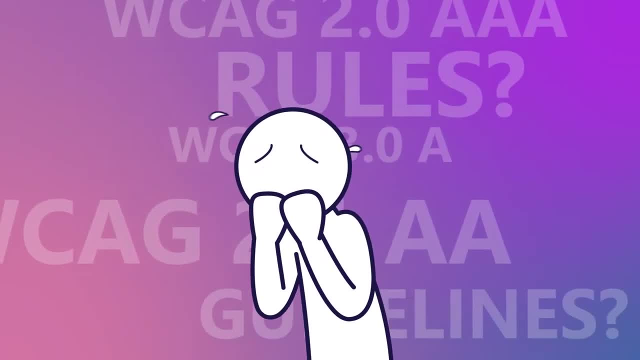 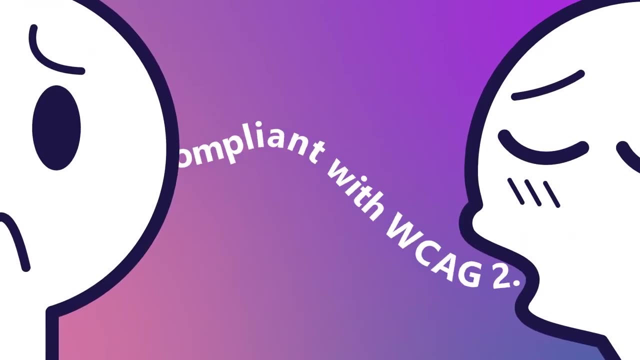 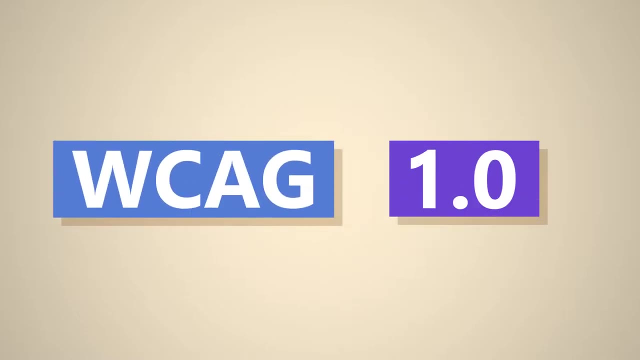 for making the web available to everyone. This may seem daunting at first, but I'm going to walk you through it. You'll often hear or see things like you must be compliant with WCAG 2.1 AA. What does that even mean? Let's break it down a little. WCAG has a standard like 1.0 or 2.1,. 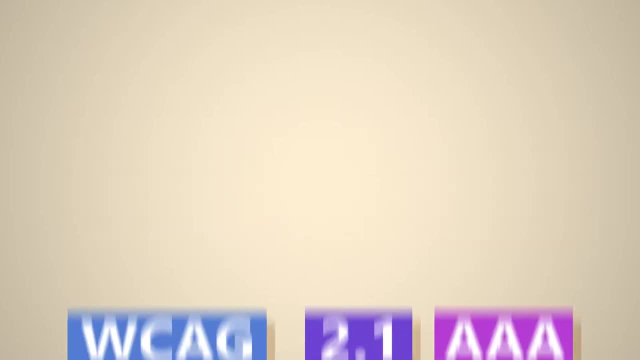 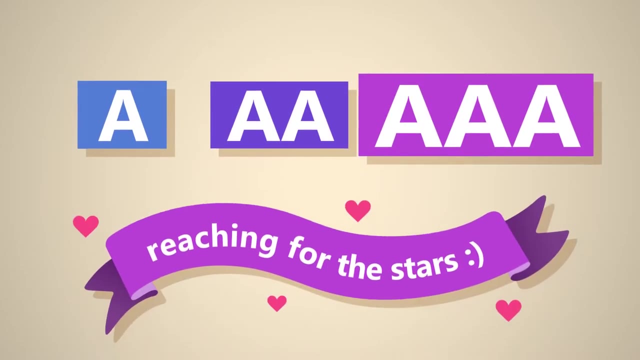 and a level that's A AA or AAA. Here at Silktide we like to say that A is must do, AA is should do and AAA is reaching for the stars. So when the legal requirement is, WCAG 2.1. 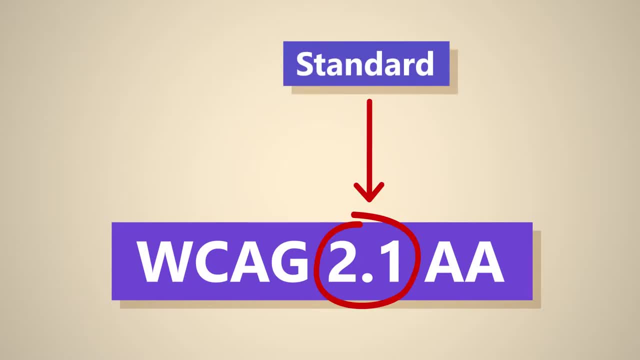 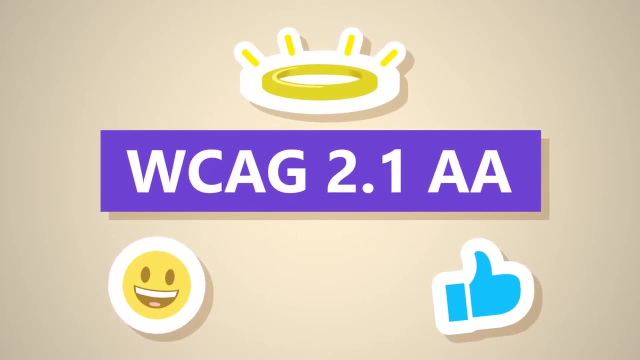 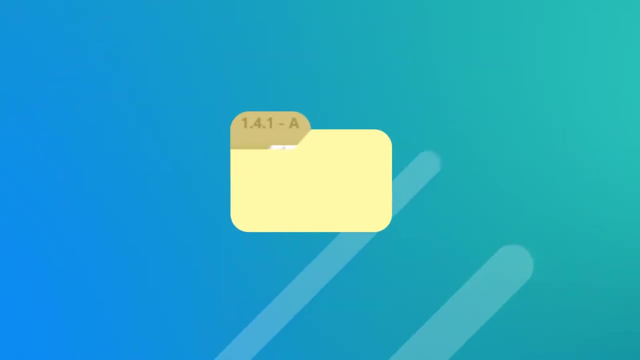 AA, it means it's using the latest standard 2.1, and level AA- the middle one, AA, is tougher to master, but still well within the reality of the web. today, All the guidelines are numbered like 1.4.1- use of color. This is a single A requirement. 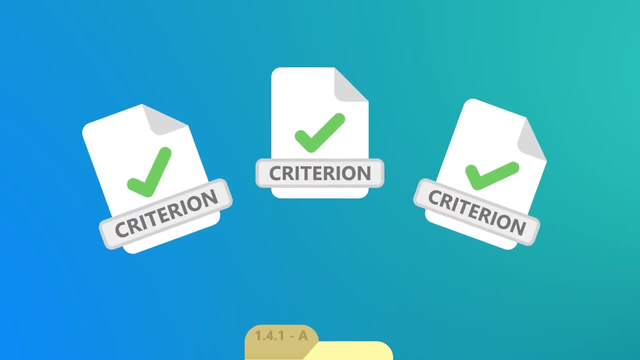 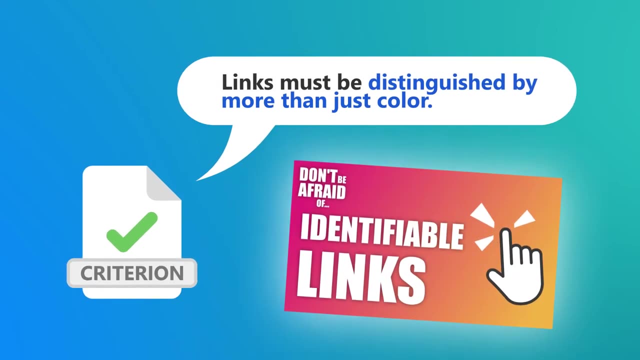 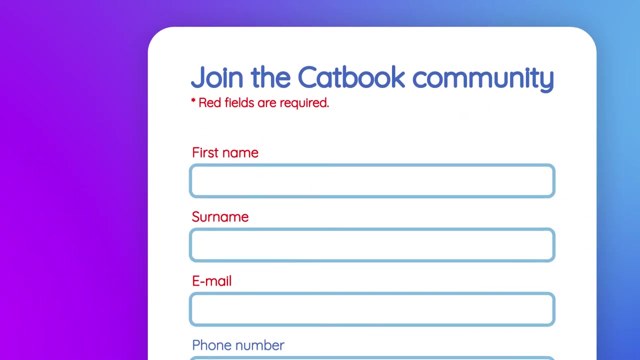 and it covers a fair bit of ground. Inside that guideline are success criteria. One such criterion is links must be distinguished by more than just color. We have a video on that topic in this series, but it also covers things like not using color for instructions like red fields or 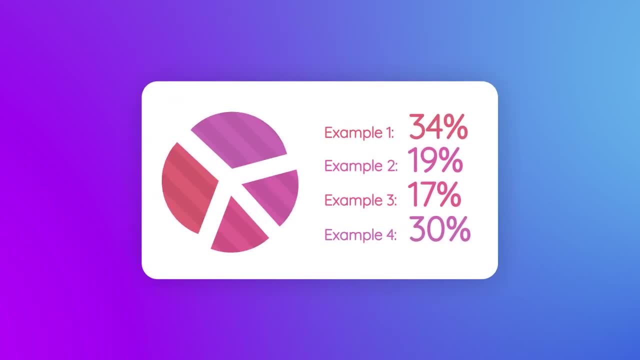 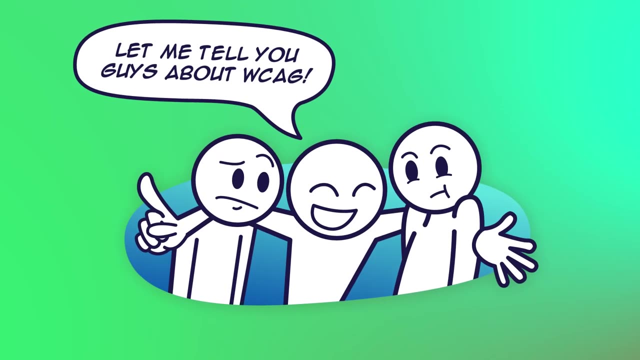 acquired, or making visuals like pie charts, with no labels or patterns to discern the segments. See, That wasn't so bad, was it? Now go tell your friends. Everyone deserves access to the internet. If you need help getting your website up to scratch, visit silktidecom.